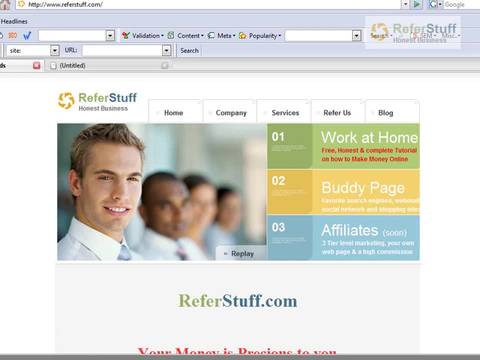 Hello everyone. this is Richard from referstuffcom. I received a phone call from my buddy today telling me that his internet provider has sent him a letter saying that some company is suing him for downloading movies off the internet. My buddy was furious because he 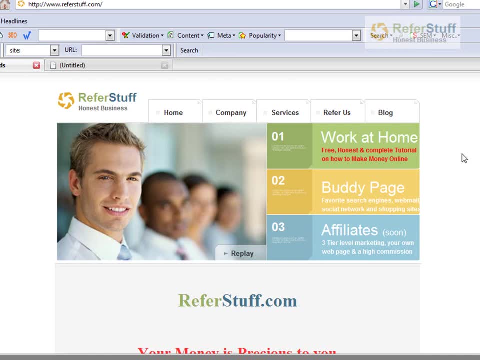 never did so and he does not have anybody at his house who does these activities. He actually has Netflix. he gets all the movies he wants. So what I did? I went over to his house to see what was going on and I looked at his internet, and what I realized is that 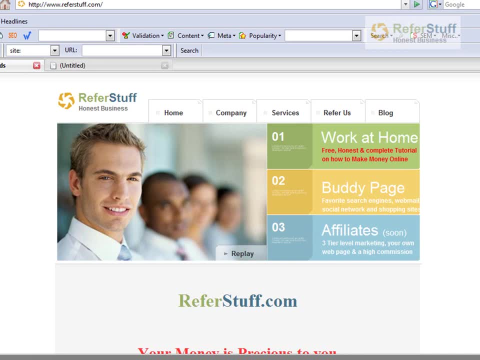 he has a non-secure wireless internet and one of the neighbors was actually using his internet connection- wireless internet connection- to download stuff using some sort of either Xtorrent or Alignwire or Emule or any of those programs. So my friend is subject for that now and he has to fight it. So I set up the security. 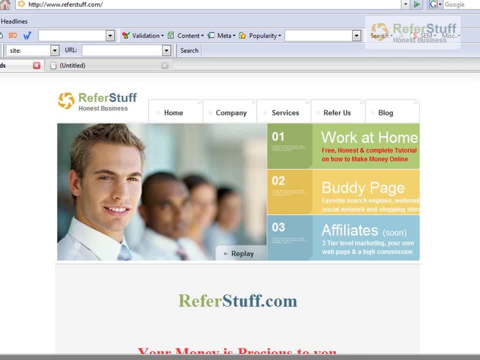 for him and I thought I really have to do this video, because there is a big problem these days. A lot of people have wireless of some sort at their house and they do not know how to secure it, and this is the big issue, And it's a very simple process actually. 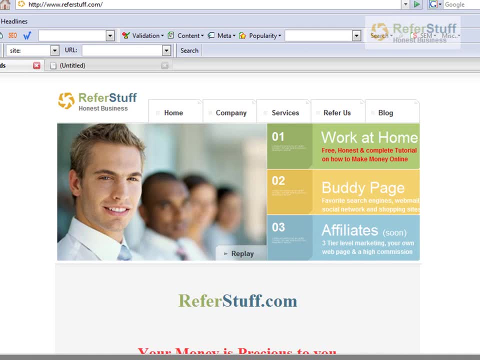 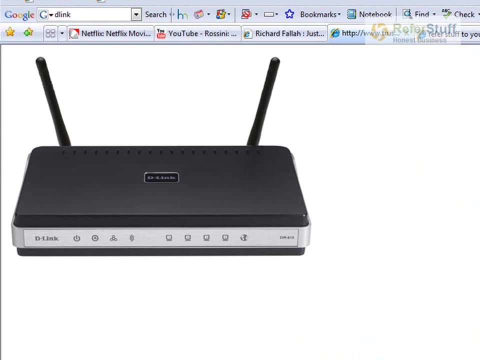 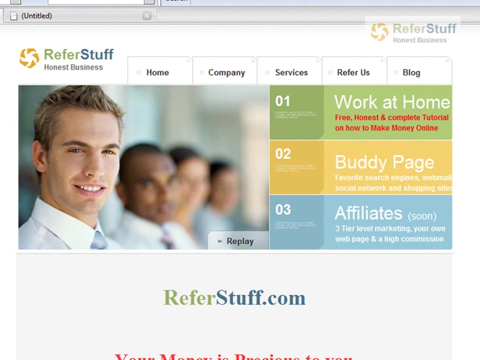 to do that, All you have to do is just flip up your router, your actual router, hold it and flip it upside down, and on the bottom of it you're going to see an address like 192.196.0.1.. Some routers might be different, but mostly this is the basic common IP addresses. 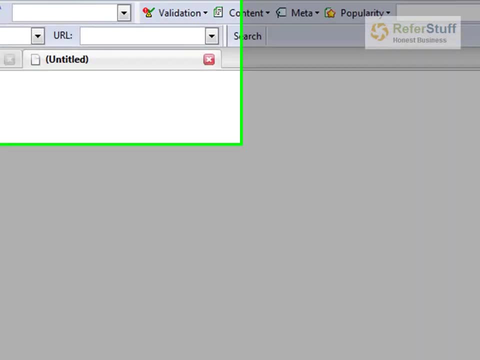 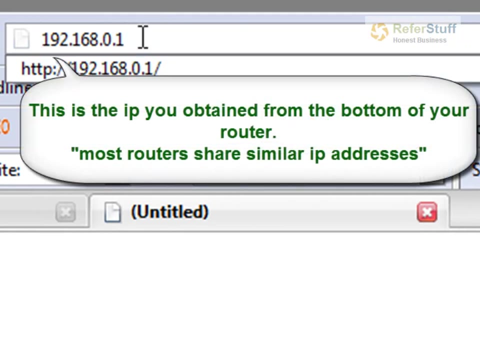 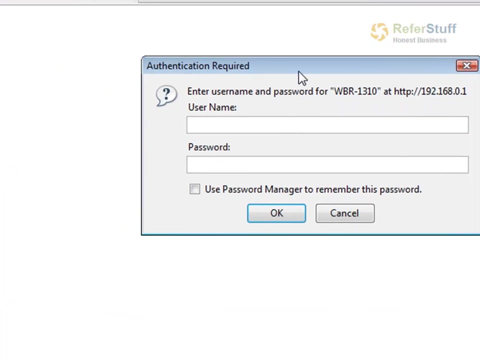 that they share. So you do that, get that number and then just go to your browser and type in that IP address- It's just as you see it right here- And then it's going to ask you for an authentication code. Now, there's always a default. If you never set it up before, there's a default. 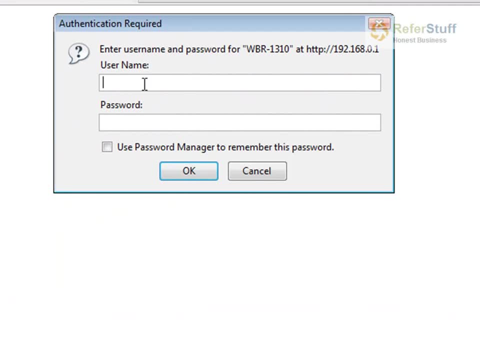 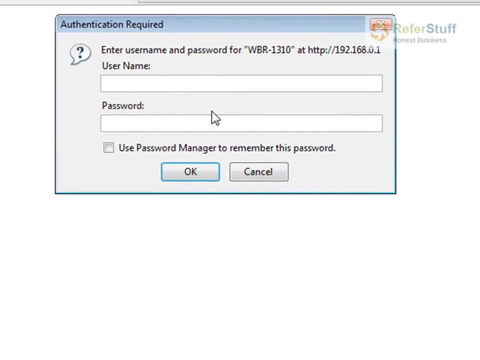 for it. Usually it's either admin admin or admin blank, or admin password, admin pass For D-Link. it's admin and then you can leave it blank, And this is how hackers actually get to a lot of places, because they know what the defaults. 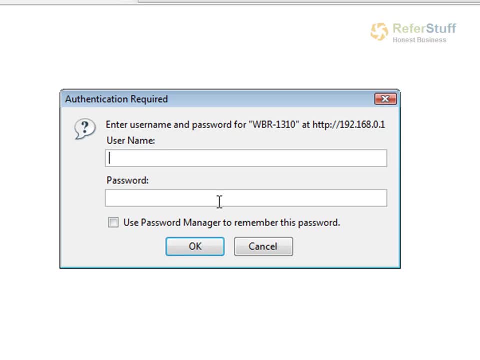 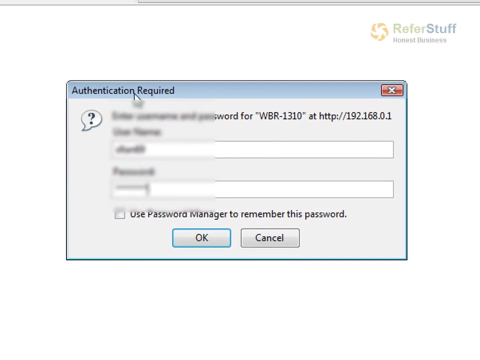 are, and they use it to get into people's business and mess up their computers and their systems. So, anyway, you put admin and you hit enter. In my case, I already have it configured, So I'm just going to put my password in my entrance and bam, you get logged in. This. 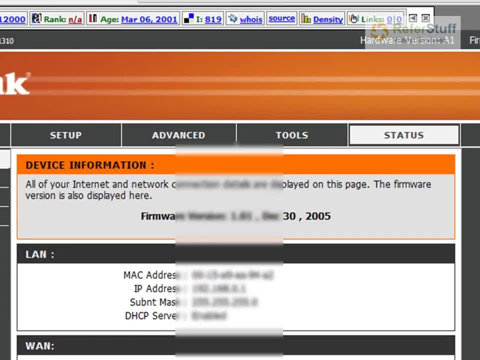 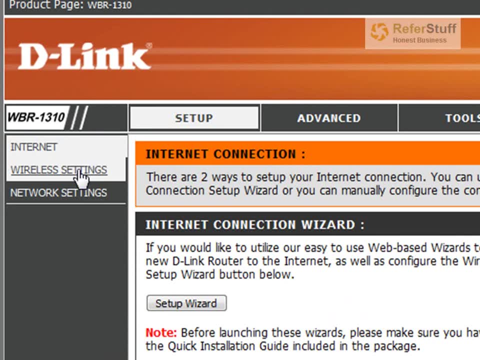 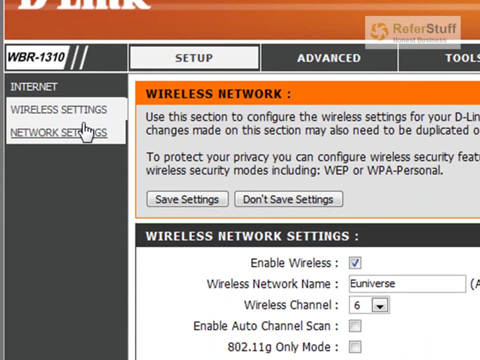 is actually the configuration page for your router, So you just go in there. As you can see, on the side you've got the wireless Click on setup wireless settings. Most of these things are really common between a lot of routers. So, again, setup wireless settings And on the bottom right here it asks you wireless. 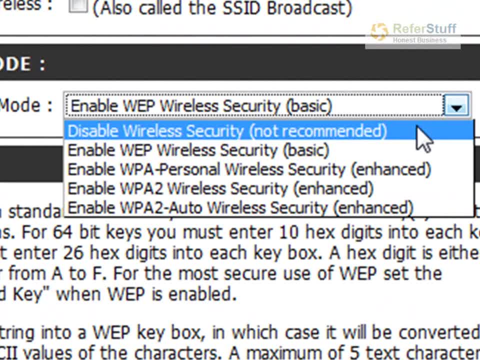 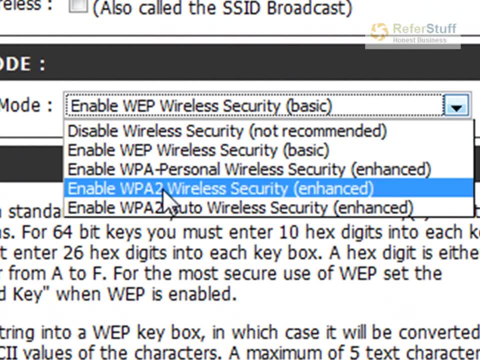 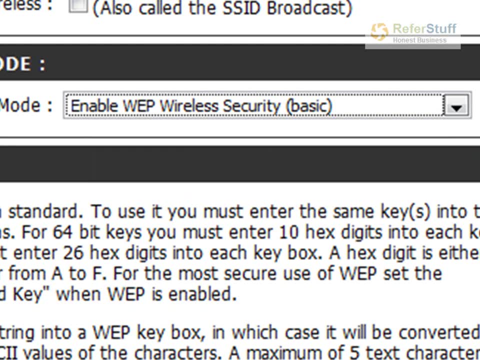 security mode. You have many different options. You can always disable it. You have WEP, WPA, which we are going to leave that for now. These are more powerful encryption but for just use the WEP wireless setting which is the basic. so you click on that on the. 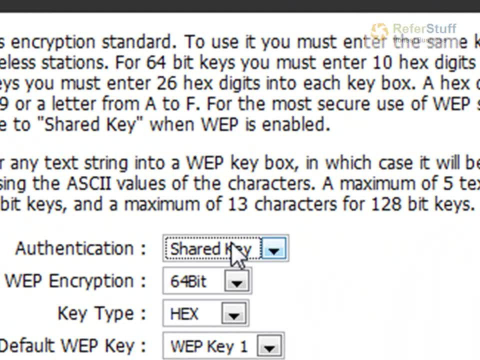 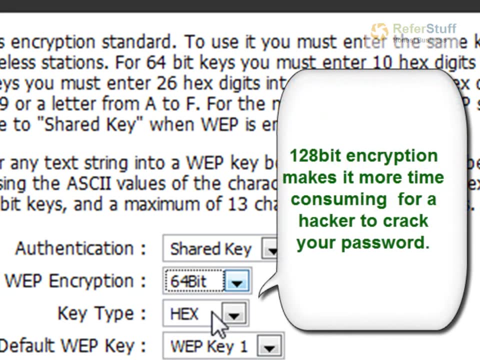 bottom. click on the share key, okay, supporting. click on the share key on the WEP encryption. it's a 64-bit. make sure you choose that, because the 128 bit you're gonna have to enter more for your password and this is gonna be really annoying for you because I think you have to pick 24 letter password and I 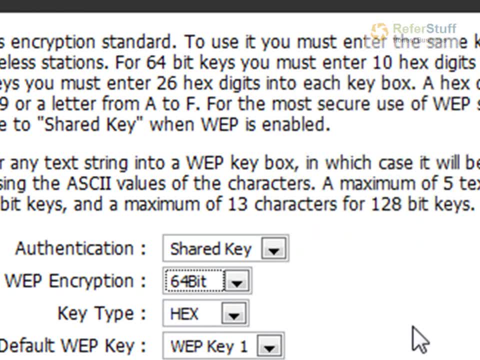 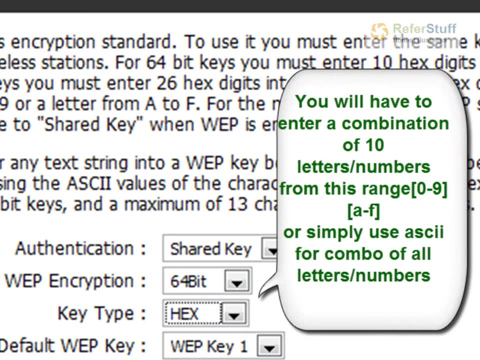 don't think you're gonna be able to remember that. if you want, you can do it. it's a stronger security, but make sure you write it somewhere and you hide it. the key type is hex, which allows you from 0 to 9 and from the letter A to F, so 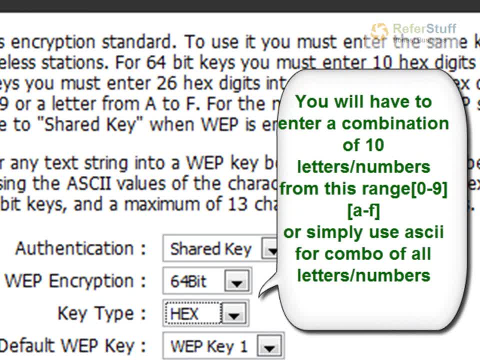 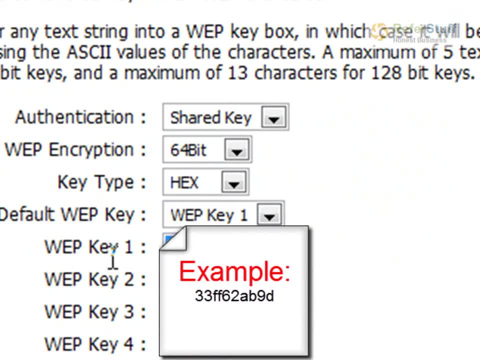 for example, your password cannot include L or N in it, or W, and then you have the default WEP, just key 1 and over here, just put in your password. you can put anything thing like, for example, 1, 1, F, F, DD, 3, 3. you're only allowed 10 in the case of 64.